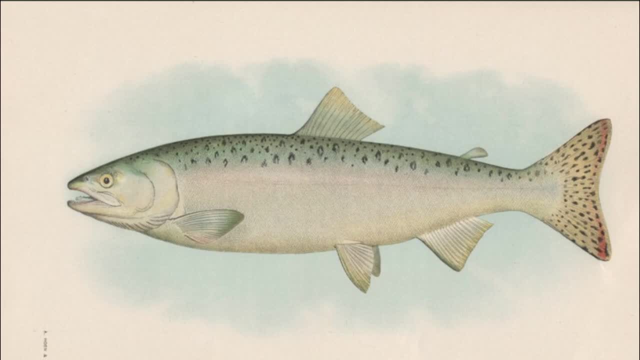 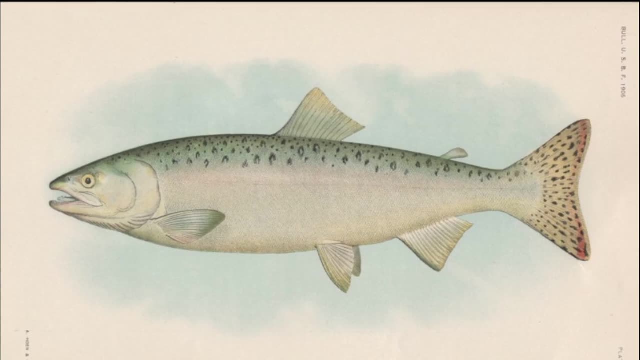 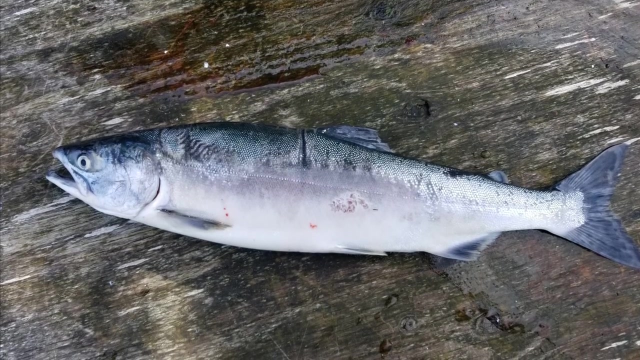 and from Russia to Korea. Pink salmon can be distinguished from other Pacific salmon by the large dark oval spots on their back and entire tail. fin In the sea. pink salmon are steel blue to blue-green on the back, silver on the sides and white on the belly. Pink salmon are anadromous, meaning that they hatch in freshwater streams and rivers, then migrate out to the ocean to feed and grow. Unlike many other salmon species, pink salmon do not reside in freshwater for a night extended period. Young pink salmon typically migrate directly to estuaries and marine waters soon after. 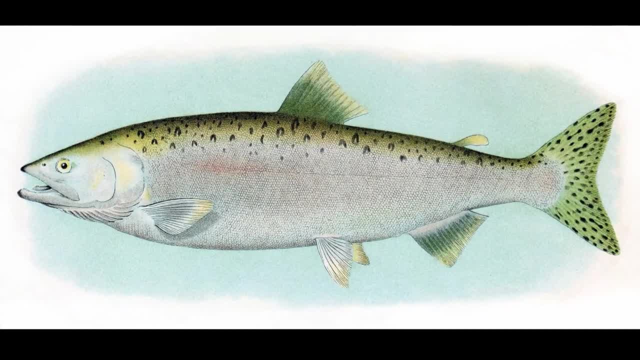 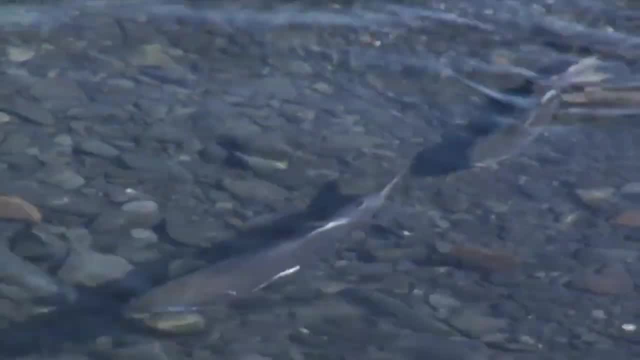 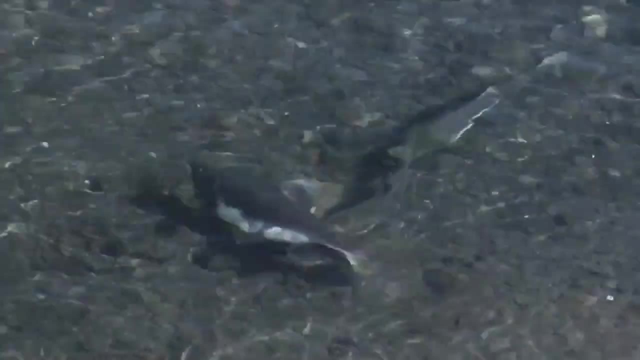 they are born. Once they reach the ocean they feed voraciously and grow quickly. After about 1.5 years of feeding and growing in the ocean, pink salmon typically return to freshwater to spawn, usually from August to October. They usually spawn in small rivers near the coast and in estuaries near the mouths of 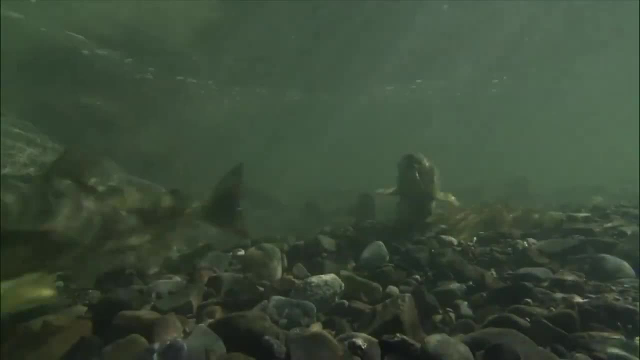 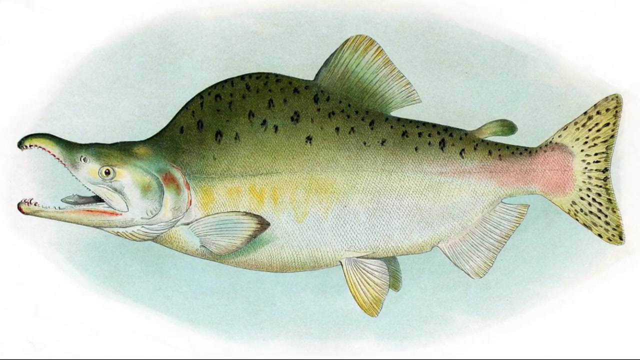 rivers. Most do not travel farther than 40 miles up a river to spawn. Breeding males become dark on the back and red with brownish-green blotches on the sides. Males also develop a hump on their head and hooked jaws. 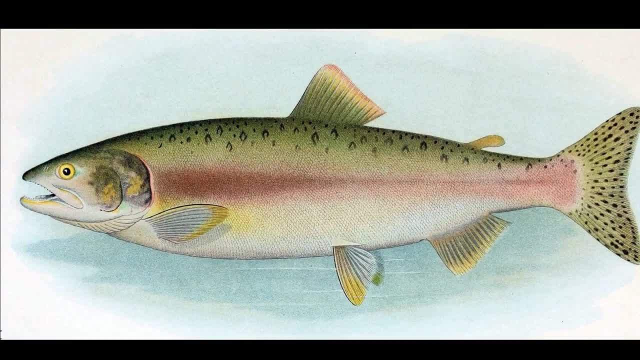 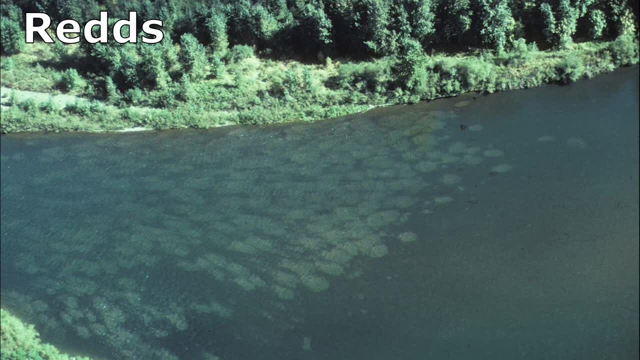 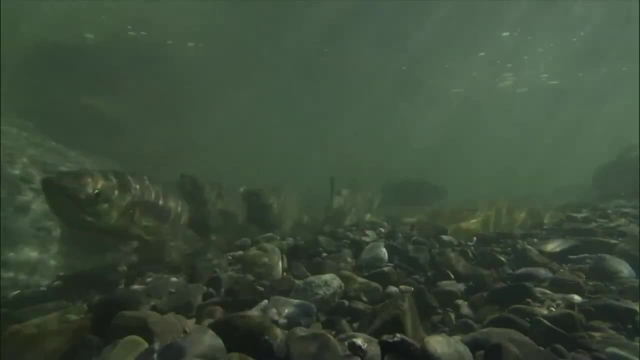 Breeding females are similar but lack a dorsal hump and are less distinctly colored. Females construct nests. They lay eggs in the riverbed by turning on their sides and digging a shallow hole. Females deposit between 1200 and 1900 eggs in the reds, which the males then fertilize. 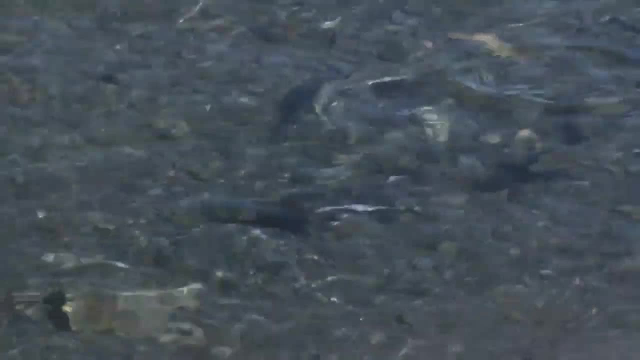 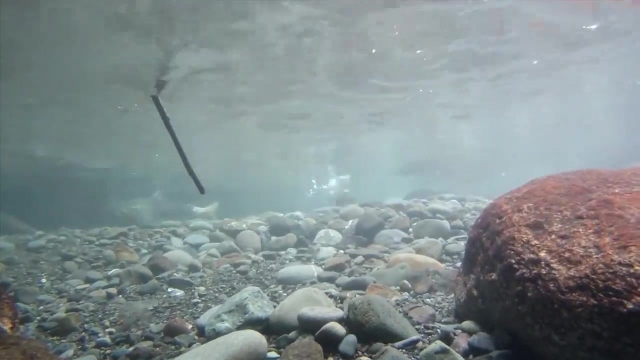 The female stays and defends her red until she dies, usually within two weeks. All pink salmon die after they spawn, making their lifespan only around two years. The eggs normally hatch during the following winter or early spring. After the young emerge from the nests, they are reared. 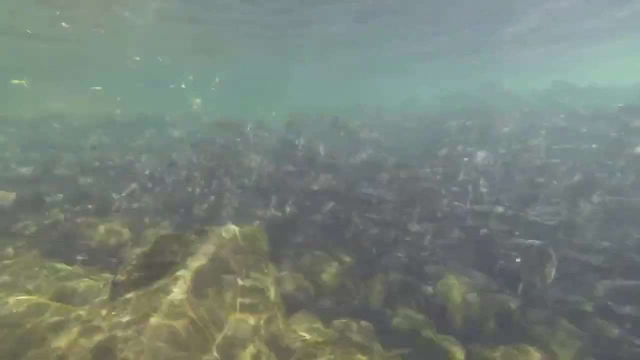 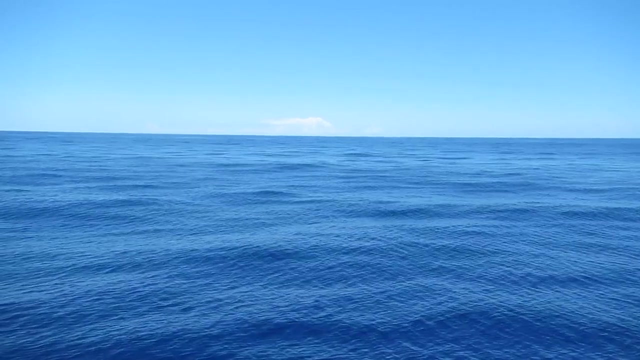 After the young emerge from the nests, they are reared. After the young emerge from the gravel and migrate, they gather in schools and remain in estuaries and along beaches for some time. Eventually they begin spending more time feeding in the deeper offshore water. 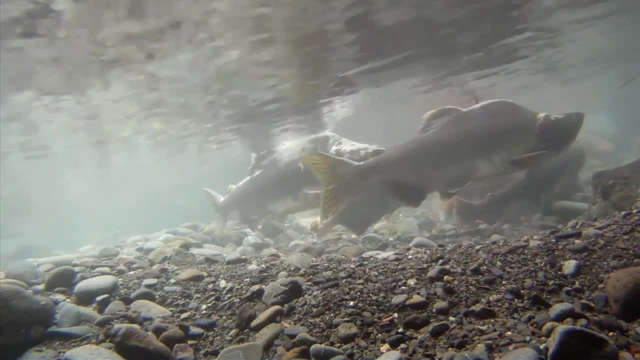 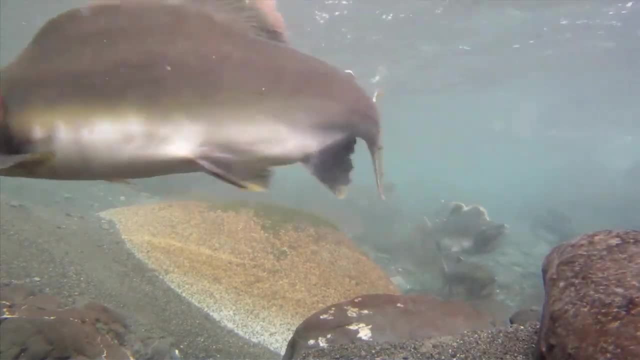 Pink salmon feed on small crustaceans, zooplankton, squid and small fish. The salmon are very heavily fished due to their high commercial value. In the 1900s, their economic value raised interest in introducing the species to new